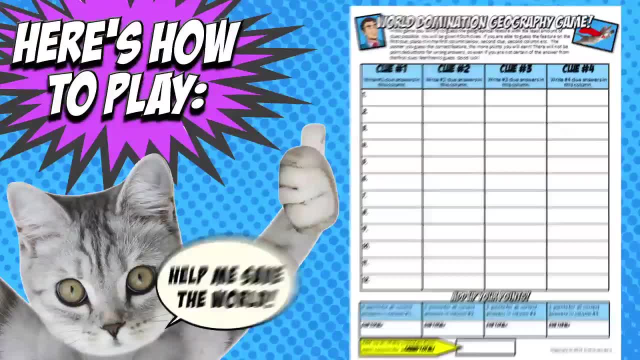 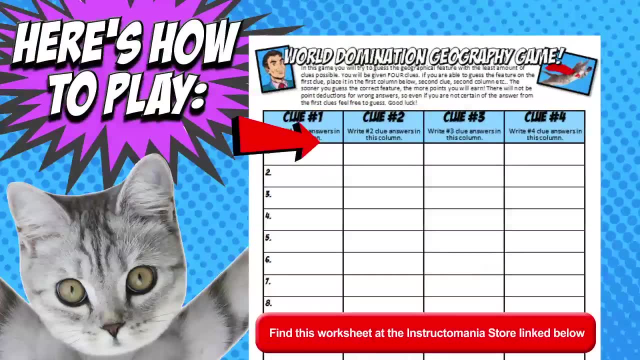 will try to guess the geographical feature with the least amount of clues possible. You'll be given four clues. If you are able to guess the feature on the first clue, place it in the first column below Second clue, second column, etc. The sooner you are able to guess. 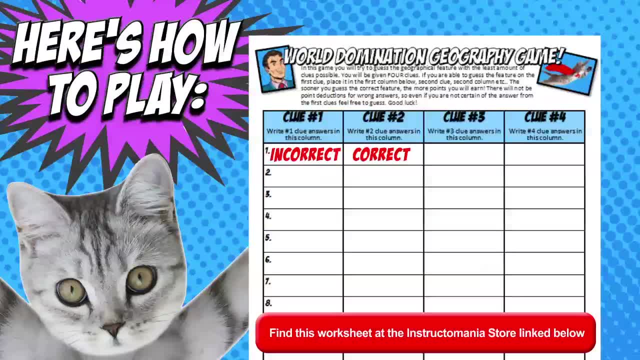 the correct feature, the more likely you are to win. In the example below, the player was able to guess the correct answer in the clue number two spot. There will not be point deductions for wrong answers, so even if you are not certain of the answer from the first clues, feel free to guess. 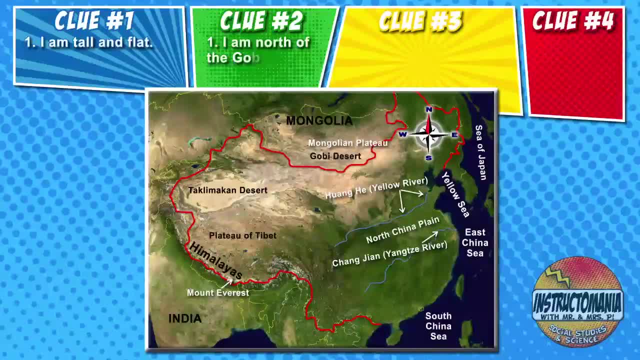 It looks like the player knows what's going on. If you've nicked the correct answer, celebrate. Make sure to give me a thumbs up. You can track any acquired or stolen information in the summary box below. Easy- See you in my next video. 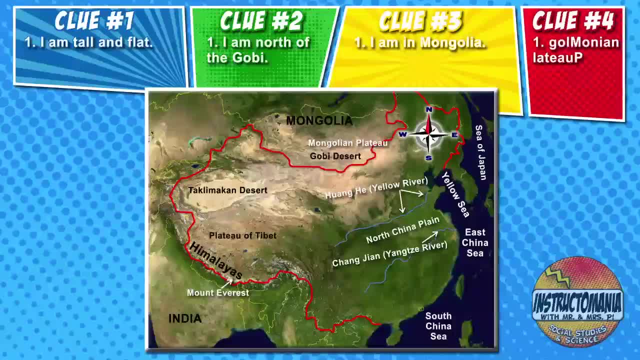 Bye, bye, Do not forget to subscribe. Do not forget to subscribe When you have a further question. like and leave a信 in the comments. Thank you for watching this video. See you in the next video. See you soon. Thanks for watching. 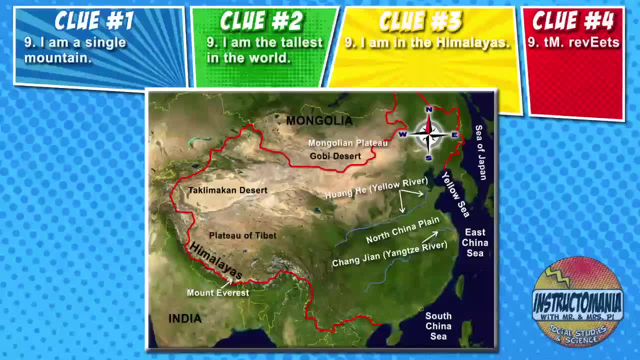 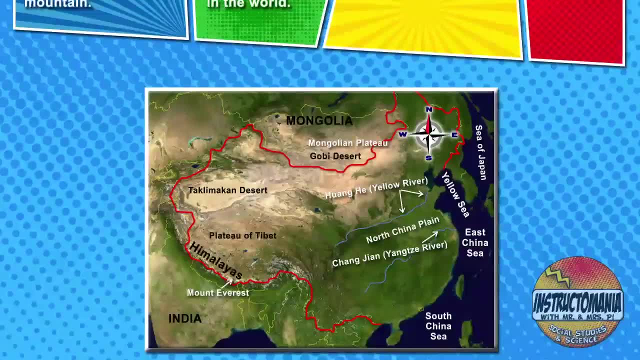 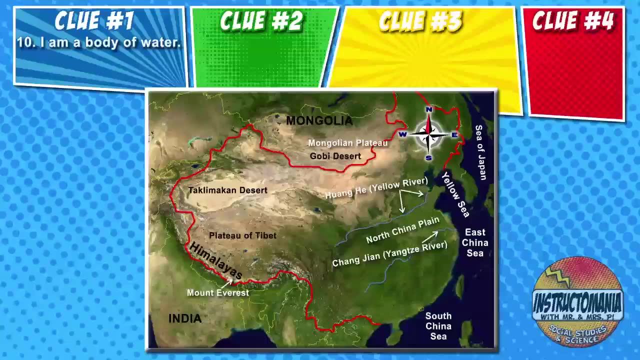 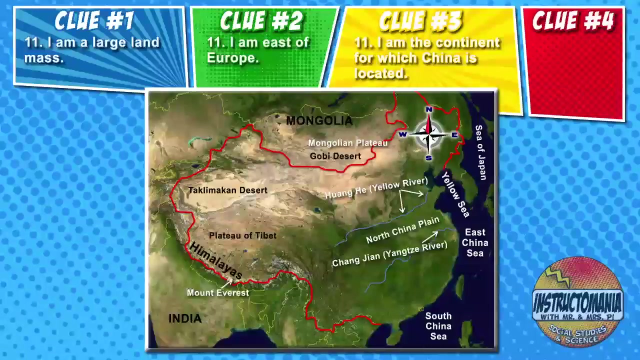 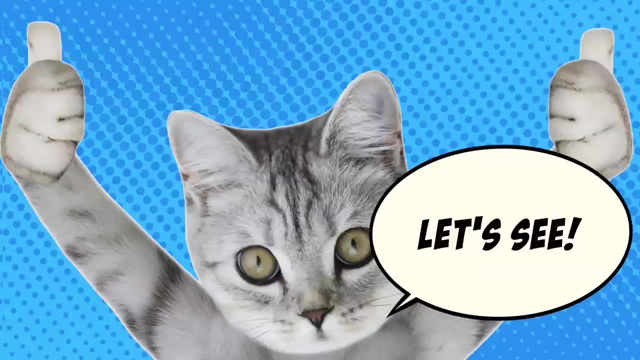 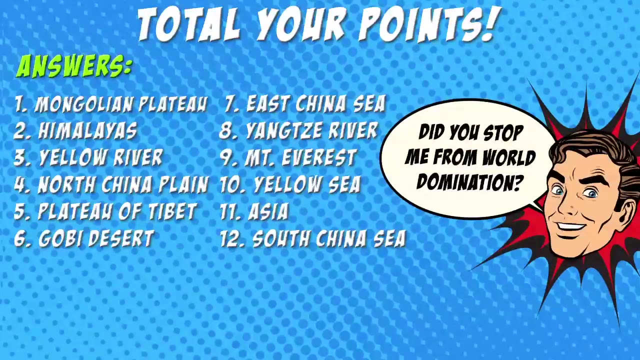 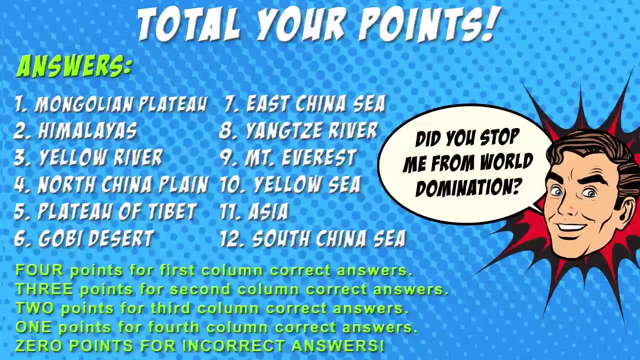 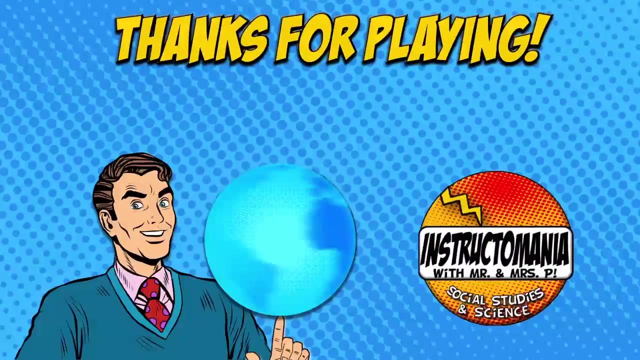 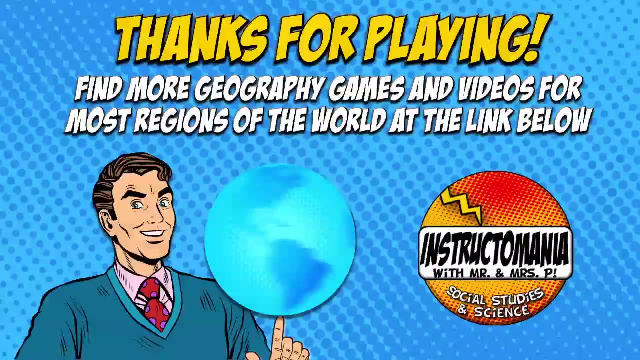 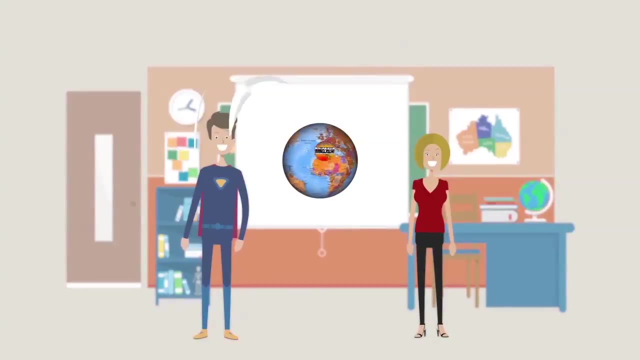